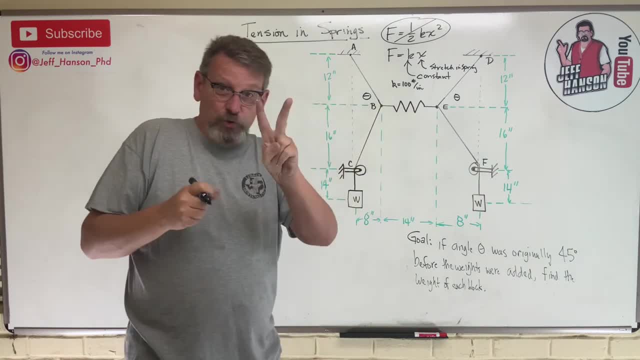 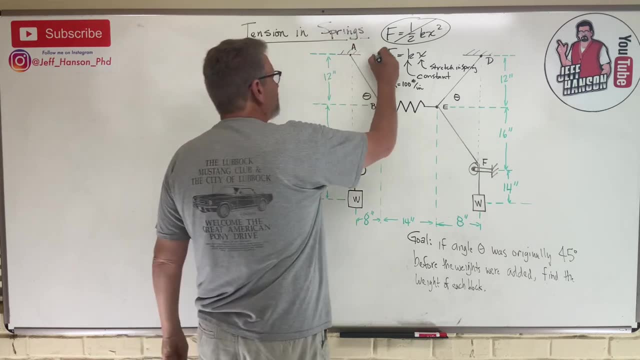 stretched, So it's now six inches. Now it's eight inches, So x would be two inches. right, It stretched two inches, okay. So that's the equation we need to go after this problem, okay. So this is that's. that's our money, right there, okay? Now what are they asking us for here? If the angle theta, which 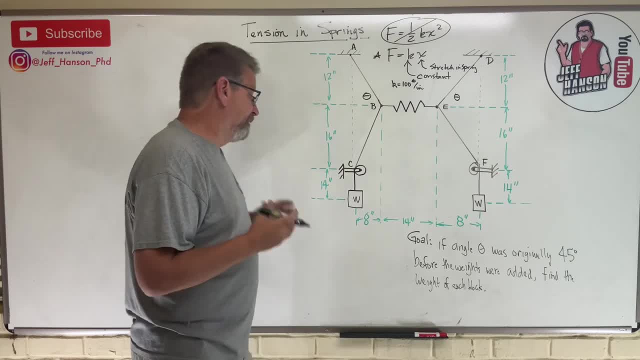 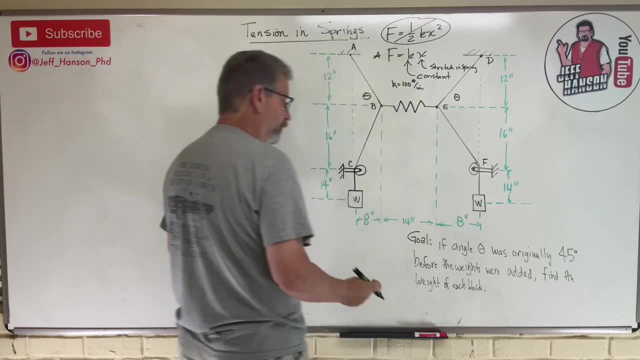 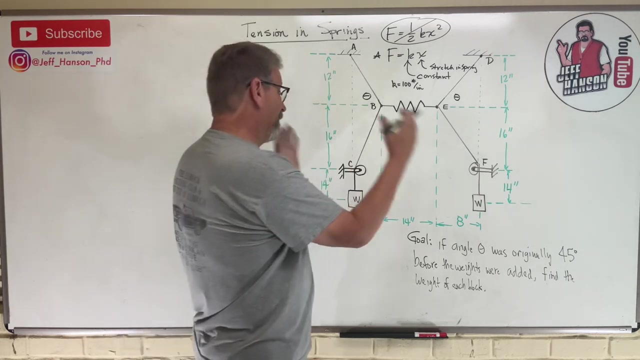 is here was originally 45 degrees before the weights were added. So, in order, and before the weights were added, these were in even farther right, Which would have drawn those weights up a little bit each block. So it was 45 degrees when it started and now that the weights have been added, this is 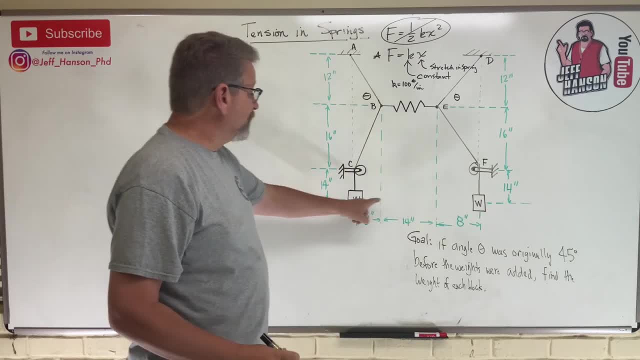 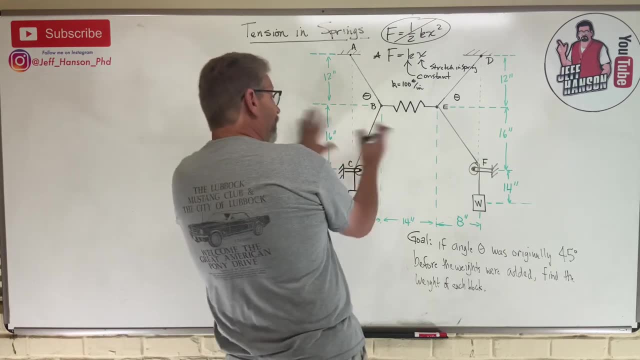 the new configuration, Find the weight of each block. Now, first thing I recognize in this problem is this thing is completely symmetric, So whatever is going on in the left half will be going on on the right half right. So I only have to solve half this problem and I think I can do the whole thing. 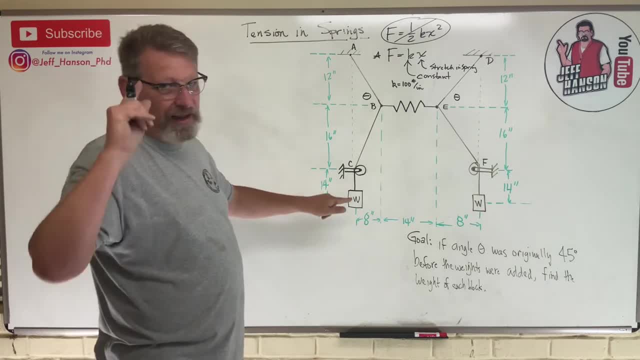 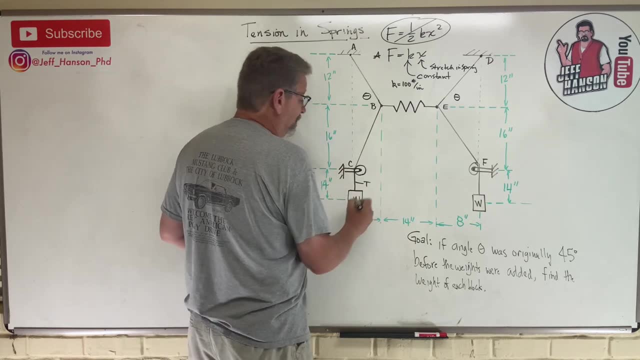 okay, So what I want to look at now. what do we know? Hey, we're pretty smart here, aren't we? What do we know about a weight going around a pulley right? That the tension on this side of the pulley is the same as the tension on that side of the pulley, right? Those two are going to be. 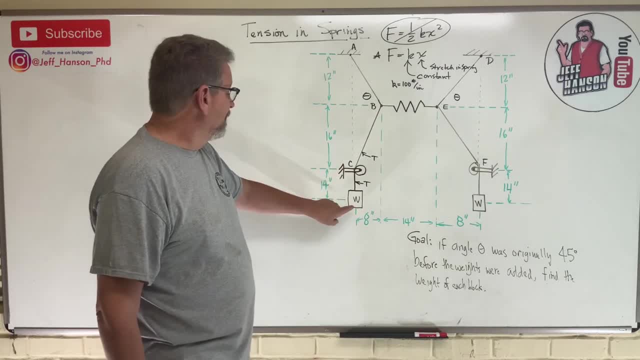 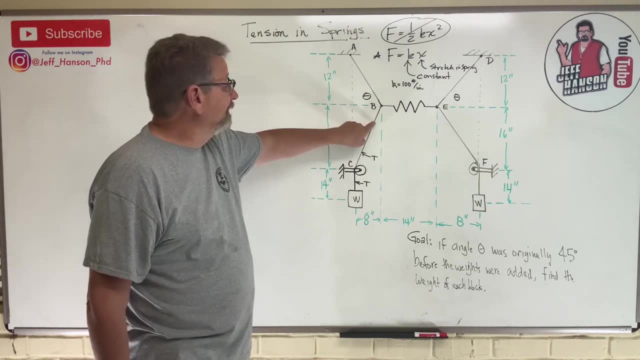 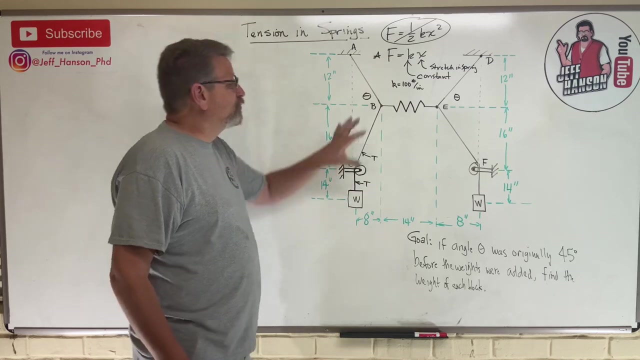 equal to each other. We know that It's a frictionless pulley, So really, if this is W, then the force in this cable here is also W, isn't it? So we start off by drawing a free body diagram, just like every good statics problem. right of joint B. Let's do joint B, You can do. 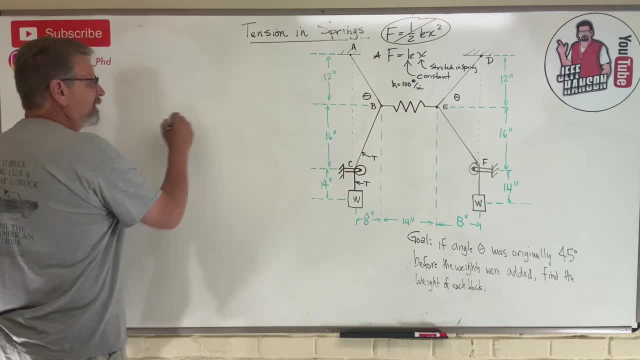 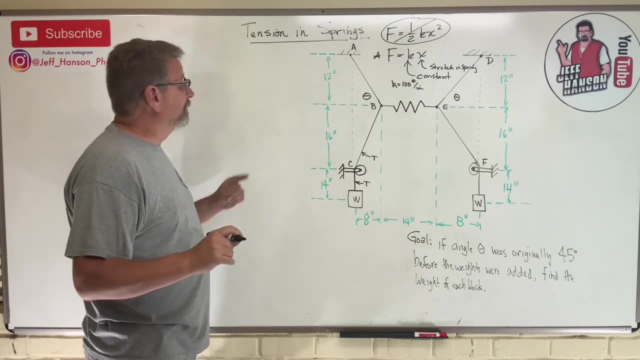 joint E: same exact thing, But we're going to do B. okay, If you're smart, pause the video and work it along with me. Skip the end, see if you get the same answer I do, but let's go okay. Joint B: What's going on? joint B: 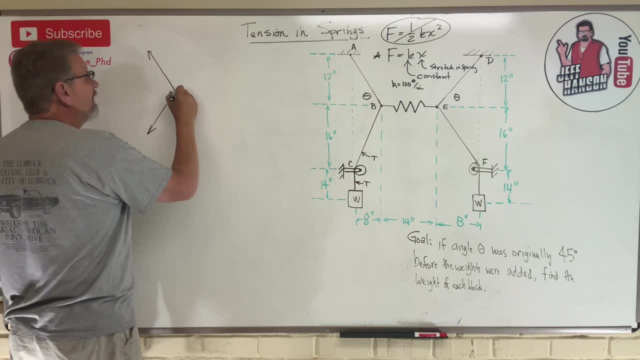 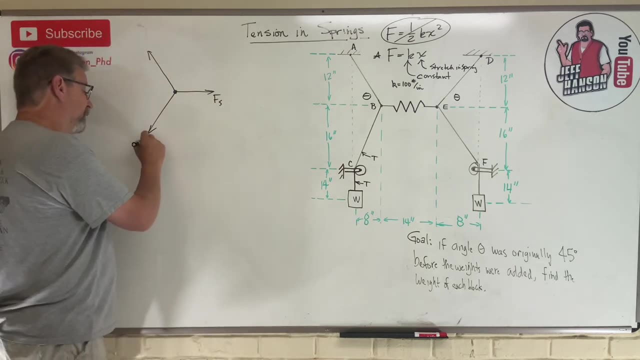 Well, I've got cables attached to me and I know that cables can only pull. Okay, I'm going to call this guy FS for force of the spring. I'm going to call this guy W- We just talked about that, right, And I'll call that guy- I don't know- FBA. 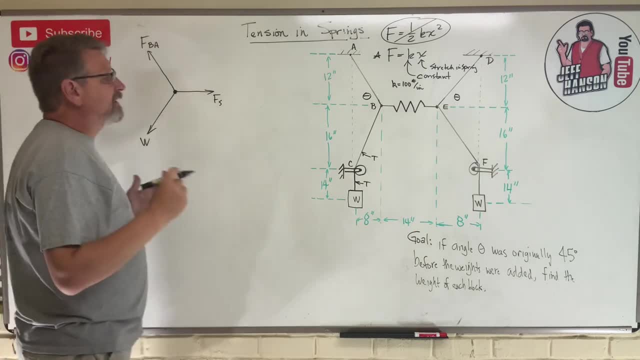 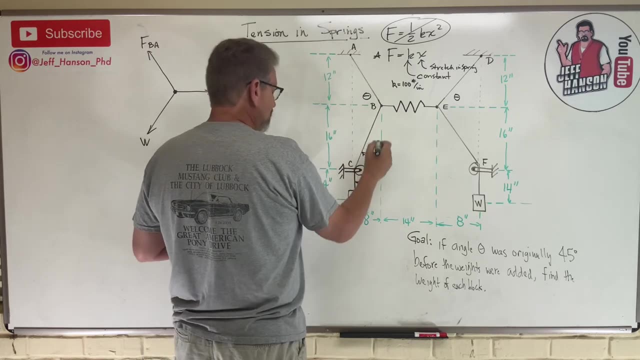 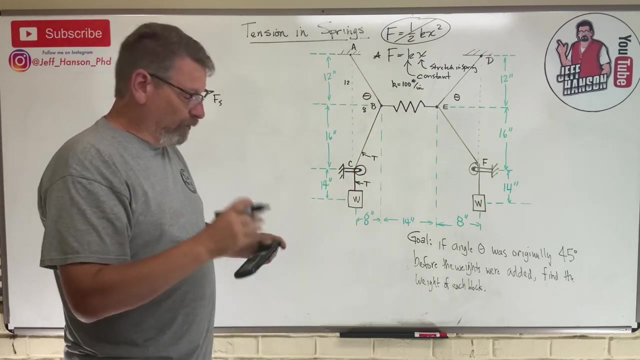 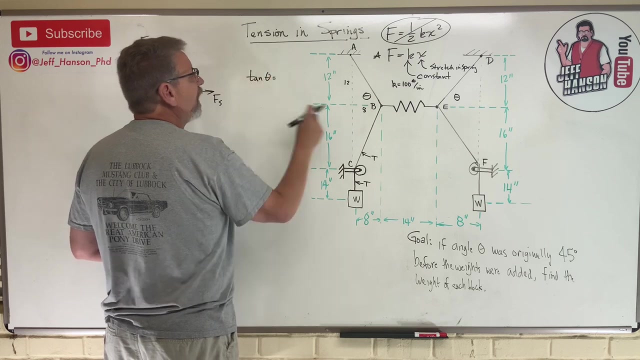 Okay, Now can we come up with some angles, Would that be okay? Okay, Now, the A is in the same line as C, right. So this little triangle right here is 12 by 8, which means my current angle theta, my current angle theta right is- I can use tangent right- 10 theta equals opposite. 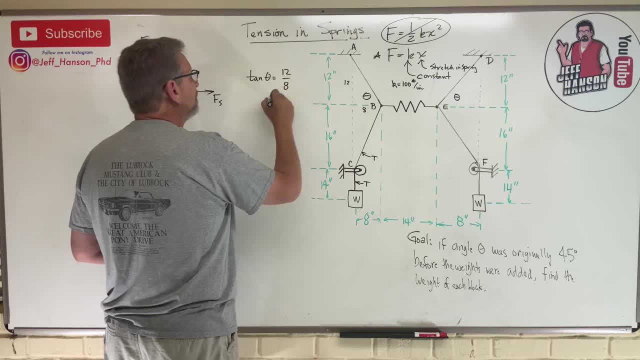 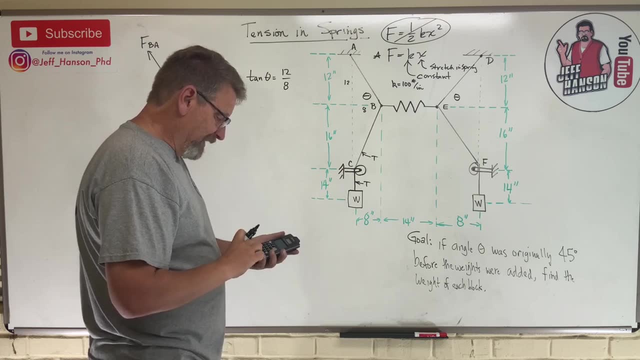 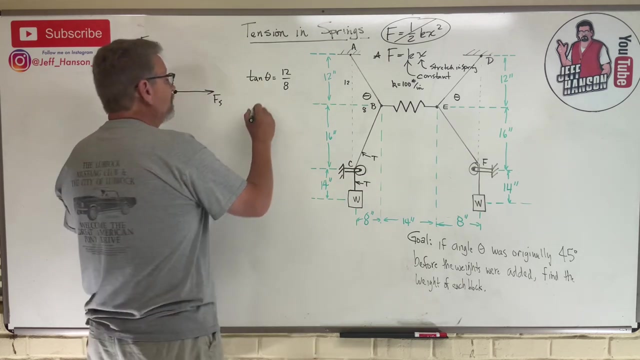 over adjacent, 12 over 8, right. Let's see what that is: 12 over 8, right, 12 over 8, right, 12 over 8, clear, clear 12 divided by 8 is 1.5, and then the inverse tan of that is 56.3 degrees. So theta. 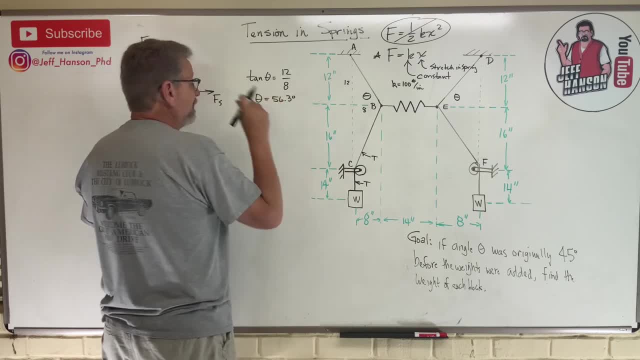 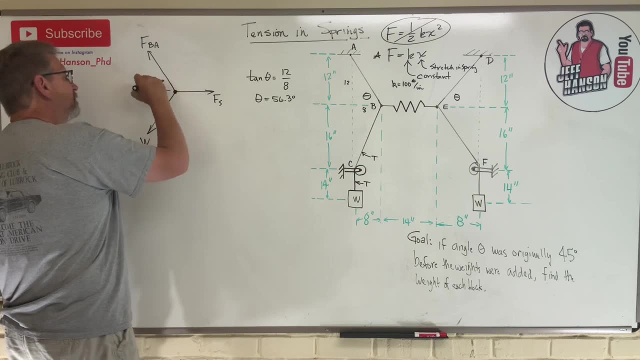 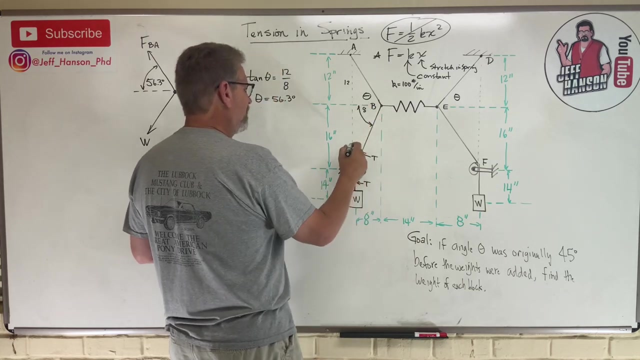 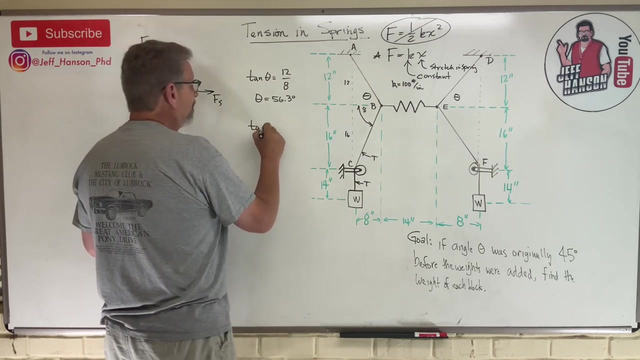 is currently 56.3 degrees. okay. So that is this angle here, 56.3 degrees, right, Okay? What about this angle right here? What is that guy? I might need to know that. Let's see: this side's 16, that side's still 8.. So that's 2, right? So tan theta tan equals 16. 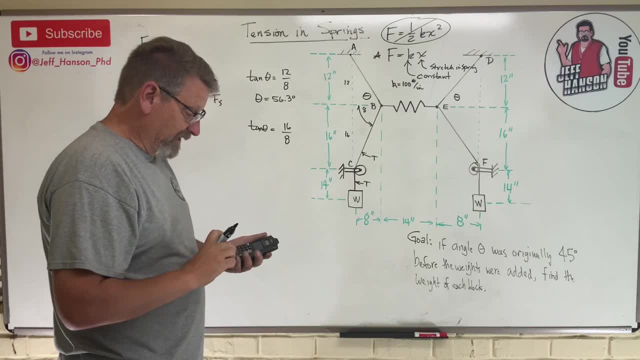 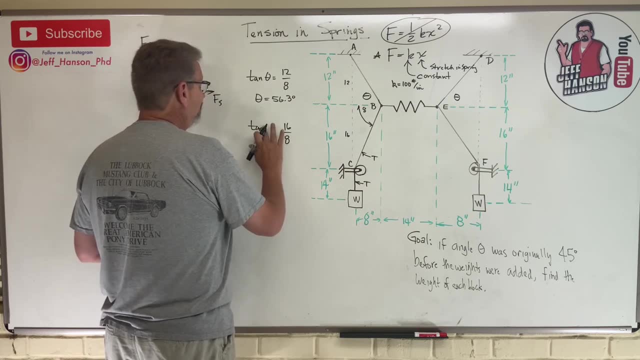 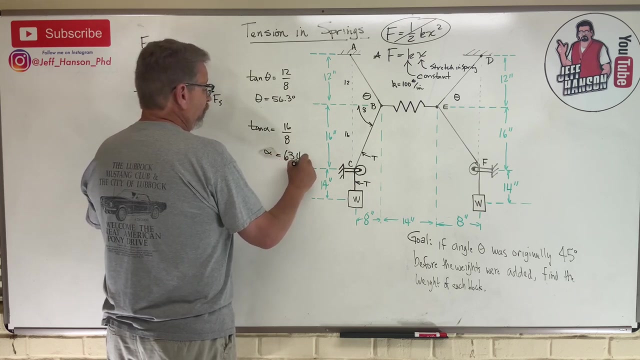 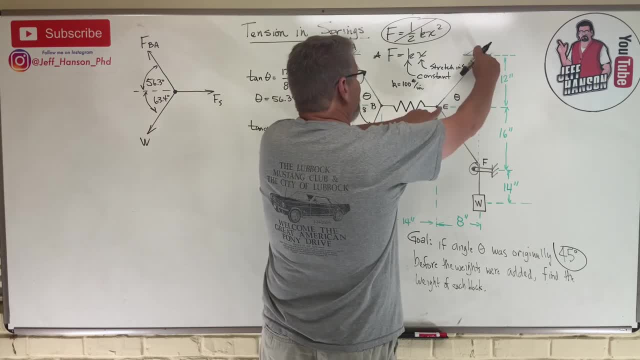 guy right here is 63.4 degrees, Okay. So this guy right here is 63.4 degrees, Okay. So this ring retracts right, This length here. this is the only thing from D to E or from A to B, that 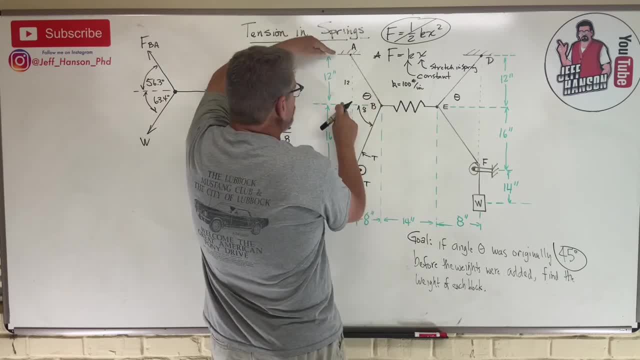 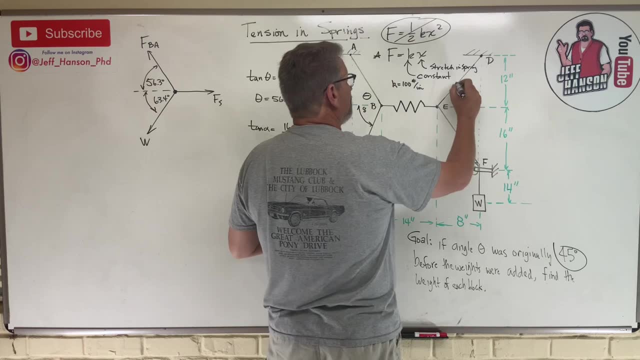 won't change, right, But this is going to rotate upwards. So 12 is going to get shorter, right, And this length down here, this eight right, is going to get longer. But what won't change is the length of that hypotenuse. Can we find that out right, quick? How about this Eight? 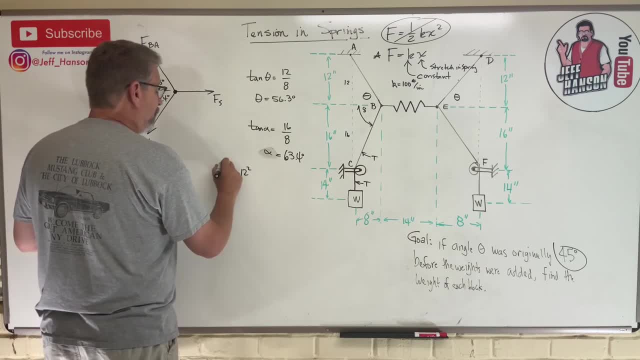 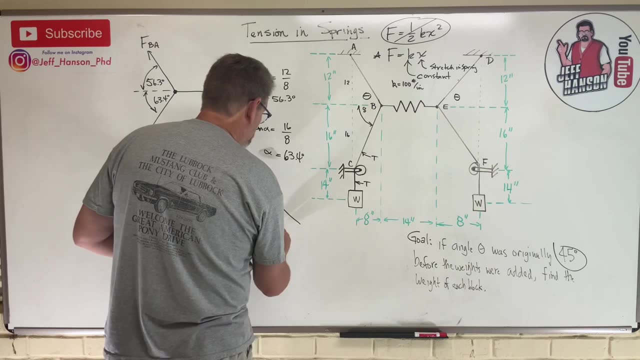 squared plus 12 squared, the square root would equal that hypotenuse, wouldn't it? Because what we're talking about? we're getting a new triangle here that looks like this: This is that hypotenuse right, Which the length will not change. 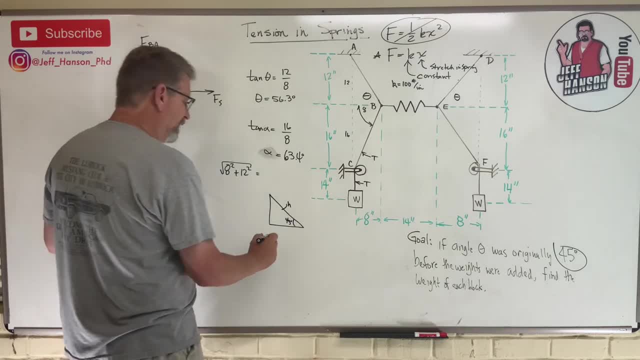 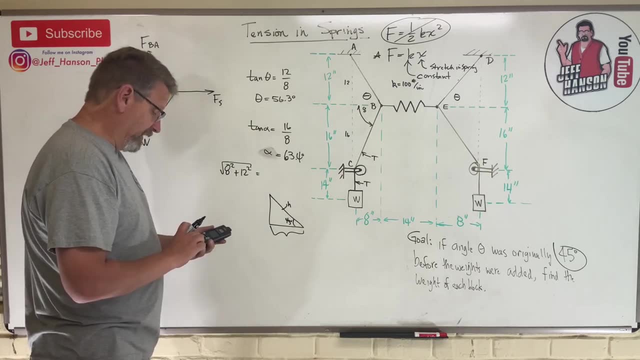 And this angle is 45 degrees, Because what I want to know is: what is this new length down here? That's what I want to know. So let's see Eight. oh, clear again. Eight squared plus 12 squared equals square root. 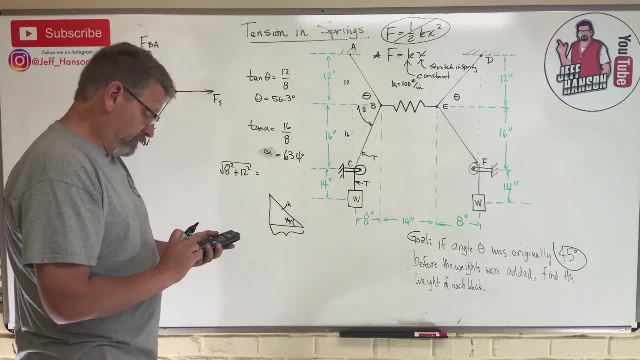 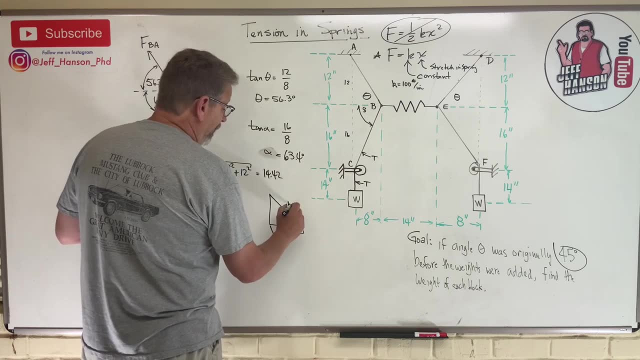 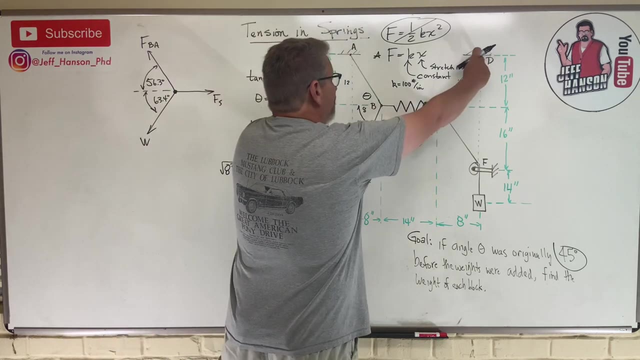 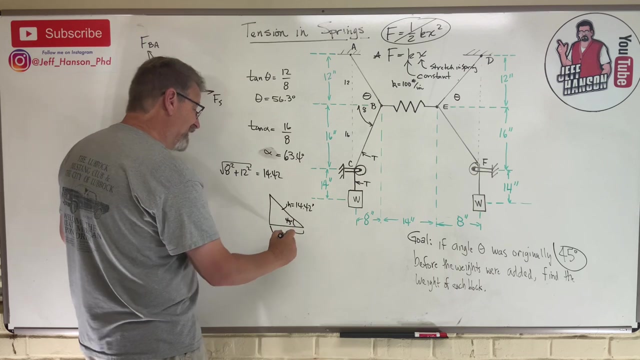 Of that equals 14.42.. Okay, So the hypotenuse is 14.42.. That's not going to change That length there or that length there, as this rotates will not change. Okay, So what is this length down here? Let's see, I know the angle. I need the adjacent side. I know the 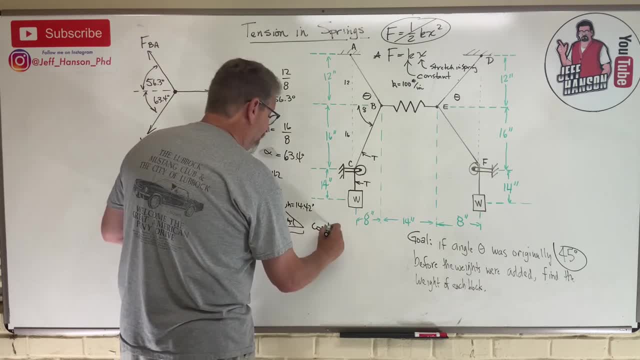 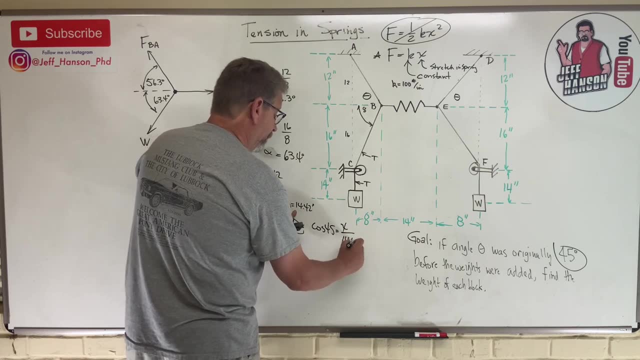 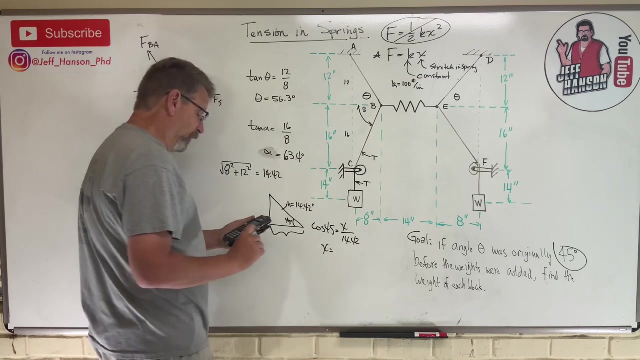 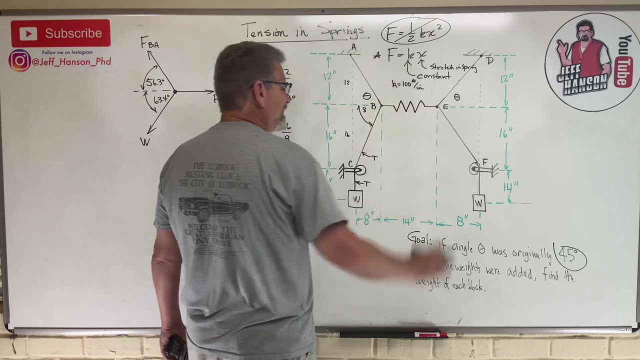 hypotenuse, That's cosine, isn't it? Cosine of 45 is equal to Adjacent, which is what I'm looking for, divided by hypotenuse, which is 14.42.. So x is equal to times. 0.707 equals 10.2.. Okay, So this length when it's 45 degrees is 10.2 inches. 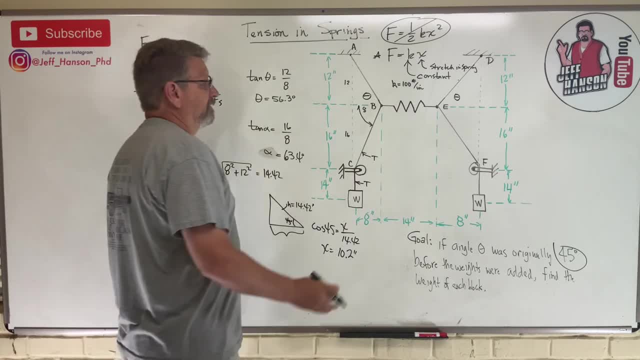 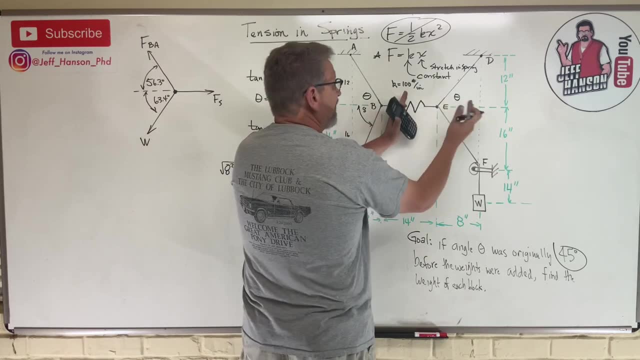 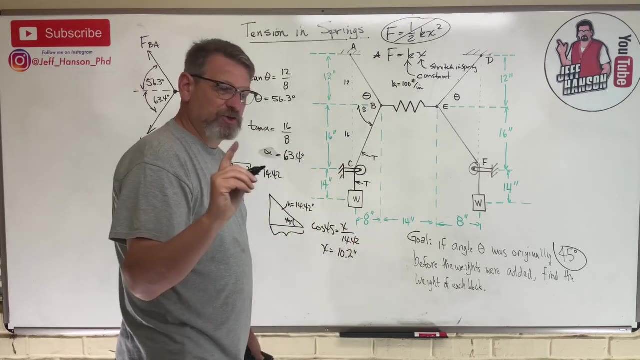 Okay, Well, if that's 10.2, it started out at eight. So how much did it? did the spring retract just on this half over here? Let's see, It went from. it went from eight to 10.2.. So how about 2.2 inches? So the spring came in 2.2 inches over here. Oh, and 2.2. 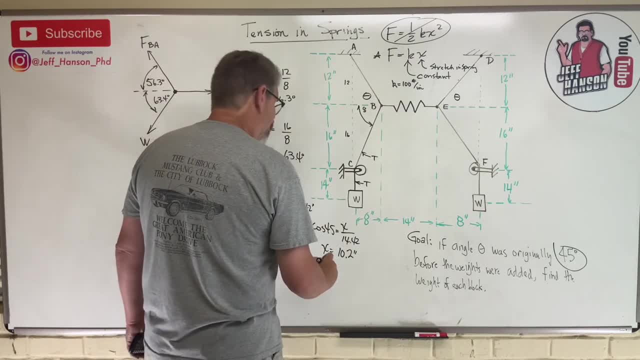 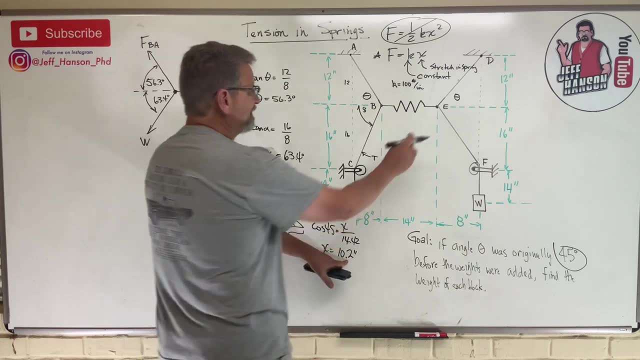 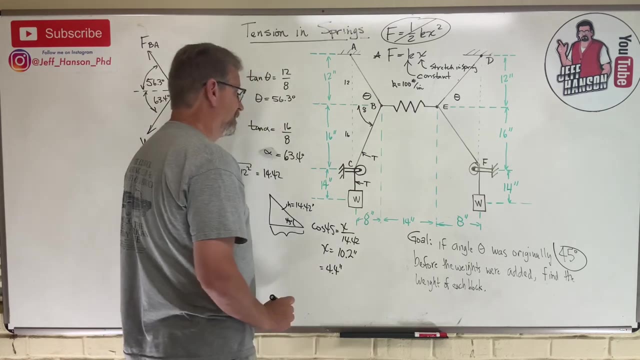 inches on that side. So the spring stretch was a total of 4.4 inches. Are you getting that? Okay, 2.2 from this side, 2.2 from that side, which is 4.4 inches. That is the stretch in the spring. Okay, Now we know the spring constant. Okay Here. 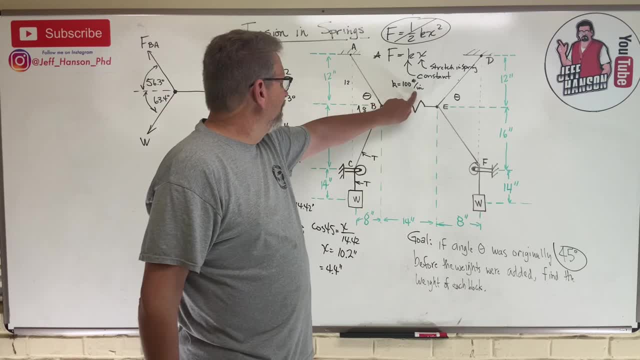 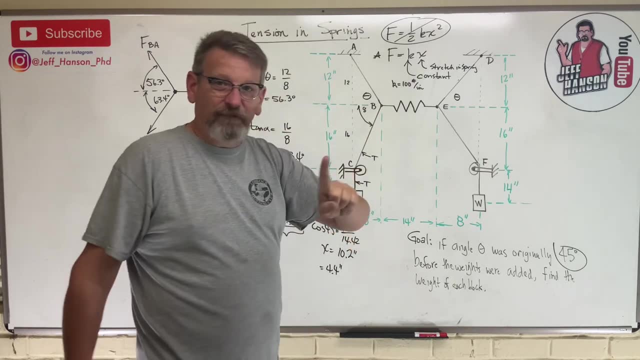 you go. Pitfall of the day. Watch out for this gang. These problems will give you this spring constant like in inches, and then give you all the measurements in the problem in feet- Watch out for mixed units- Or in newtons over meters, and then give you all. 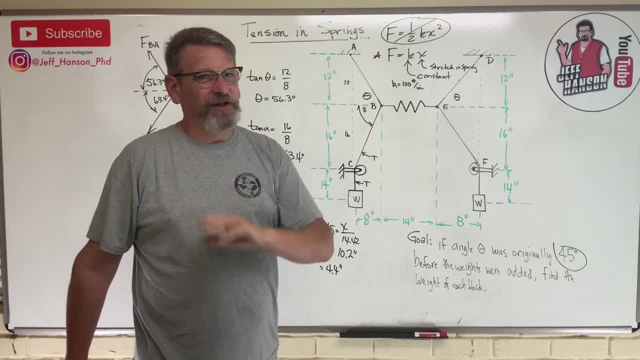 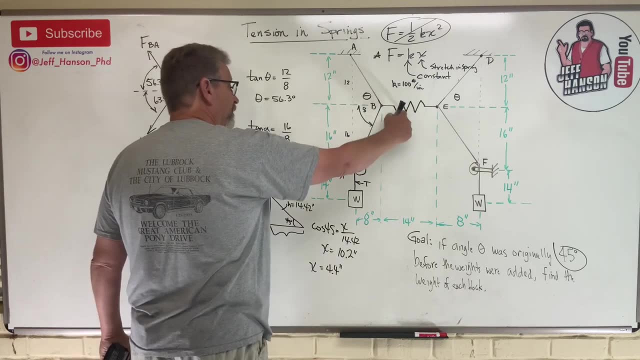 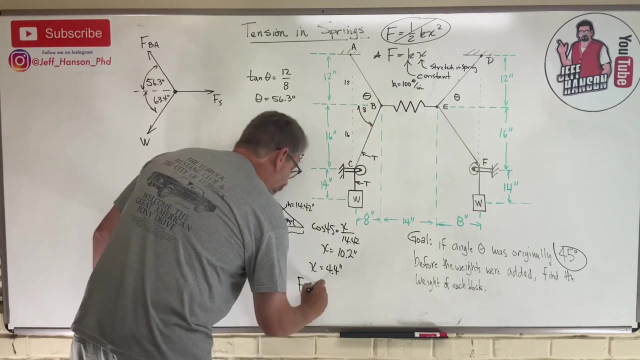 the dimensions in millimeters. Watch for, don't, don't fall for that trap. Okay, Okay, 4.4 inches. Let's use this equation to come up with a force in that spring. So F is equal to K. Now this one doesn't have mixed units, does it? 100 pounds per inch times 4.4 inches? 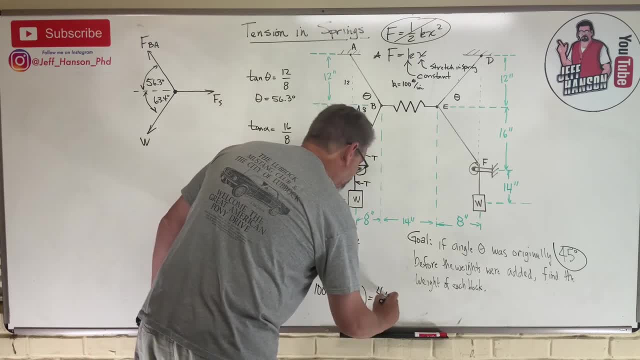 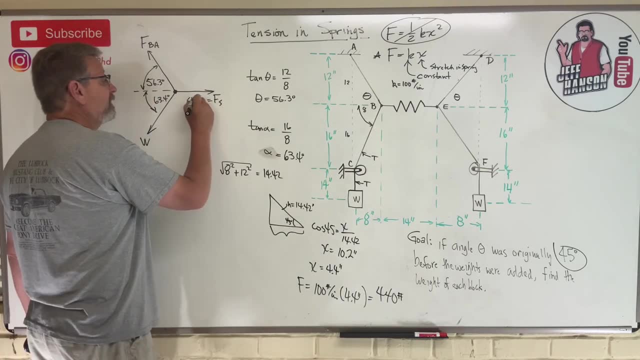 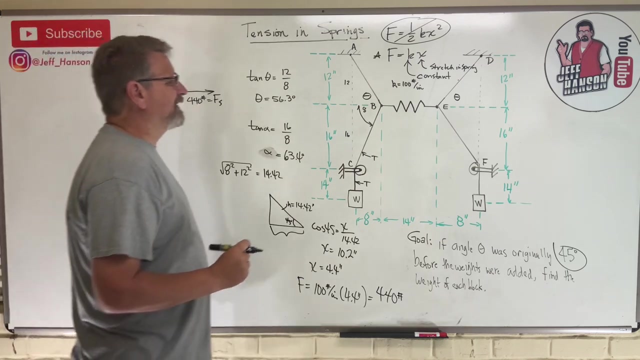 equals, I got it 440 pounds. Okay, So that is the force in the spring. Okay, 440 pounds. Okay, Be careful on that man. That's, that's tricky, You know you might say, oh, that 12 never. 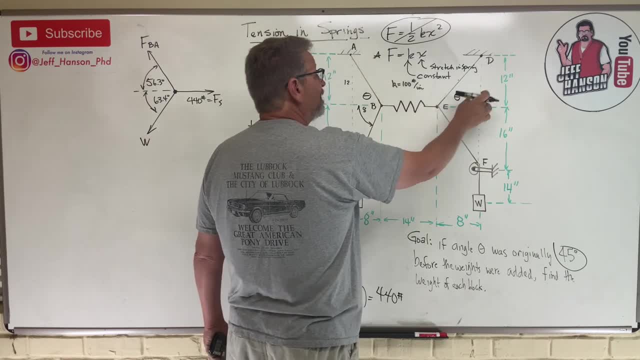 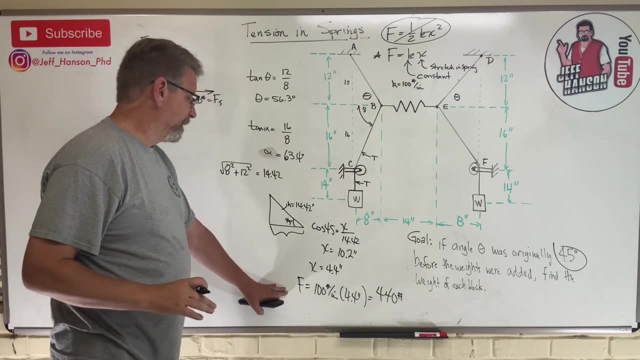 changes. so this guy goes to 12 when it's 45. But it doesn't That. that link there is the only thing that remains constant. Be careful about that. I hope you followed that. Okay, Where all that came from. Okay, Now that I know this. now, what do I have I got? 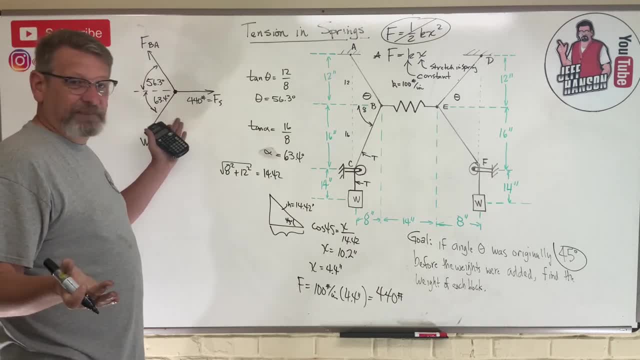 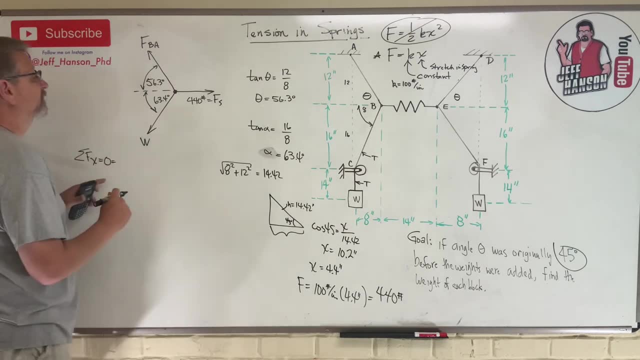 the world's simplest statics problem here from last chapter, right, We should be able to solve this right. Some of the forces in the X equals zero. What do I have in the X direction? Well, I've got 440. Okay. And then I've got minus FBA. 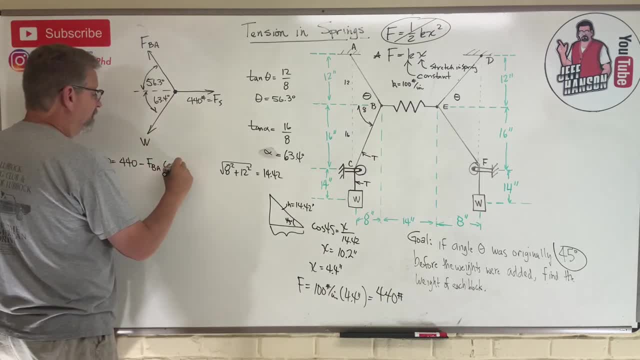 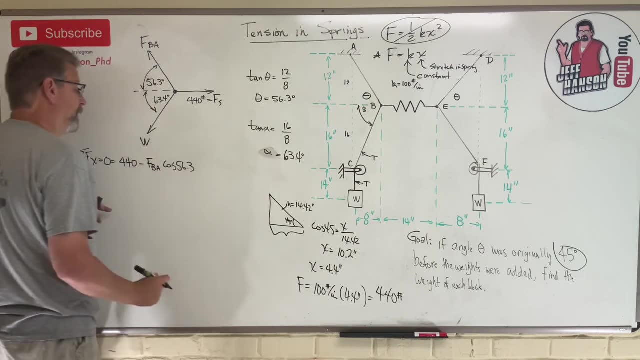 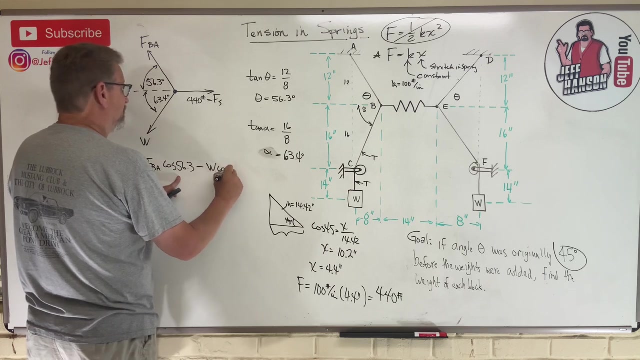 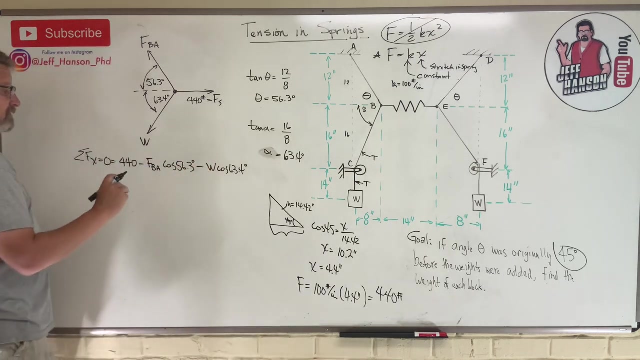 what Cosine 56.3, right, I'm erasing this. Okay, That was my hypotenuse, Minus the cosine of this one, this guy here W cosine 63.4. Degrees. Okay, There's one equation. Now let me just, let me just rewrite that equation. 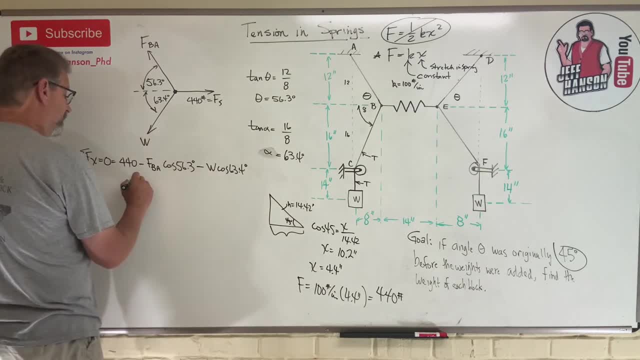 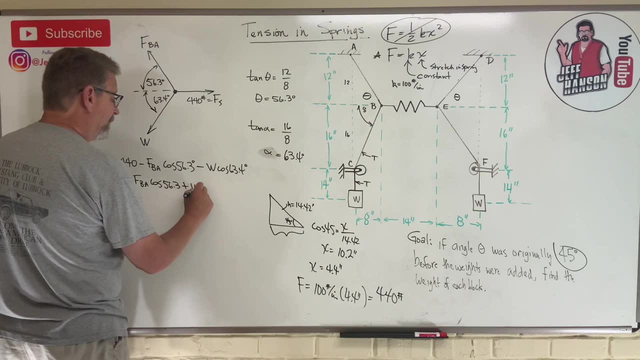 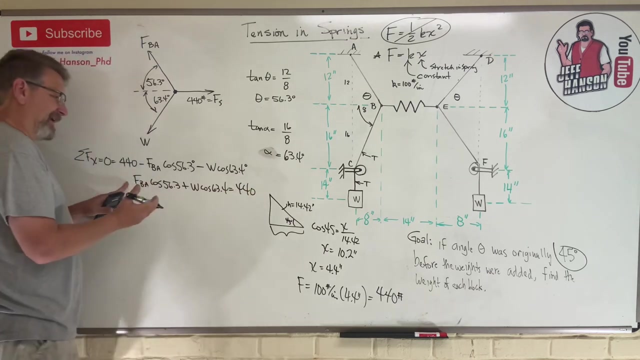 I'm going to take these two negatives, move them to the other side. I'm going to get this: FBA cos 56.3 plus W cos 63.4 equals 440.. Okay, Just rearrange that equation. You know why. 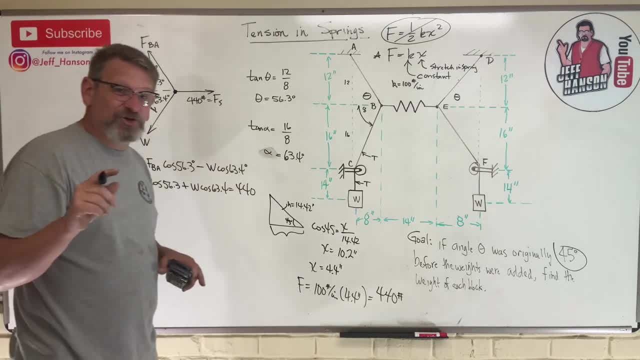 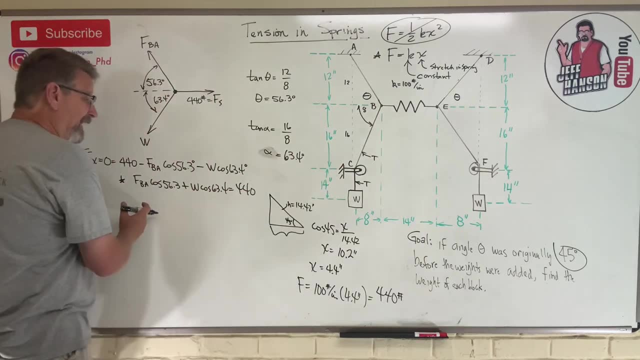 Because this equation has two unknowns. I bet my Y equation is going to have two unknowns in it, which is a perfect job for my system solver. You could use the substitution method and a little bit of algebra, but you know, when you've got a calculator that'll do it and it. 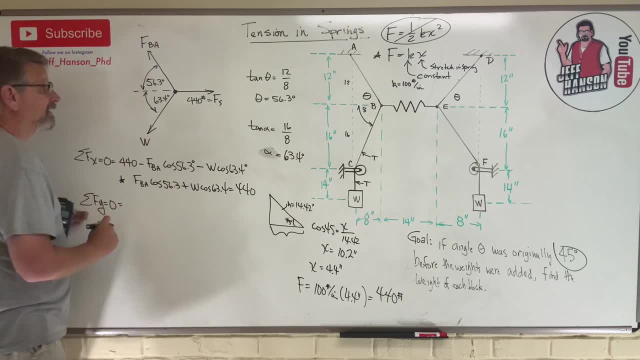 doesn't make algebra mistakes. that would be would kind of be silly to do, wouldn't it? Okay? So the last equation is this guy, I've got FBA going uphill times the sine of 56.3.. Okay, Yeah. 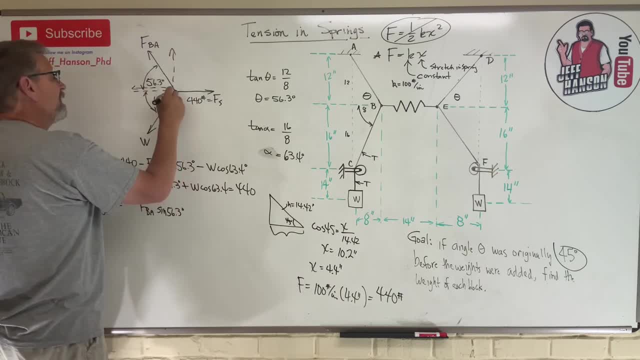 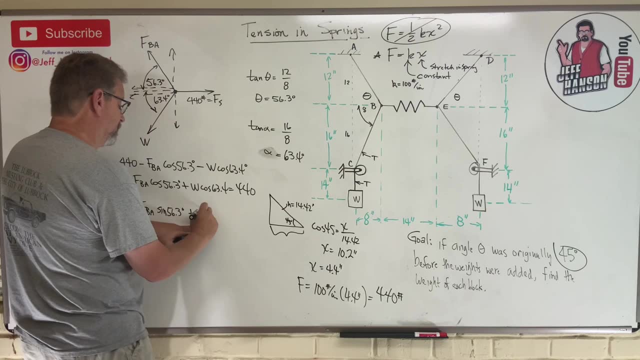 Just remember, these guys have components here and here And here and there. That's what we're doing, is we're? we're adding those components up, right? So plus W sine, Oh, not plus. He's going downhill, That's a minus. 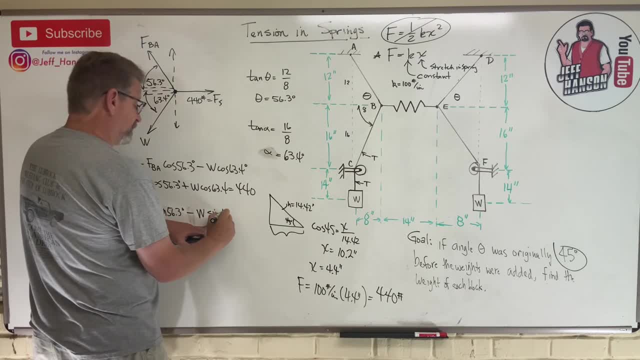 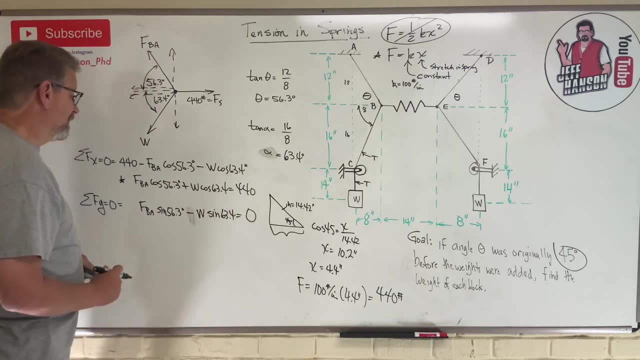 Dr Hanson, you almost messed that up. Okay, 63.4 equals nothing else in the Y, So a big fat zero. Okay, So again I have written. I've got my two equations here and I have written them in columns. 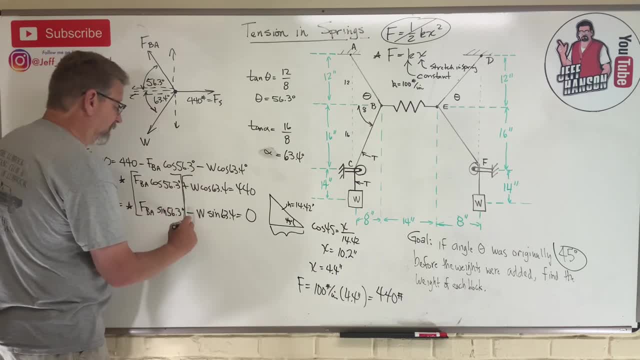 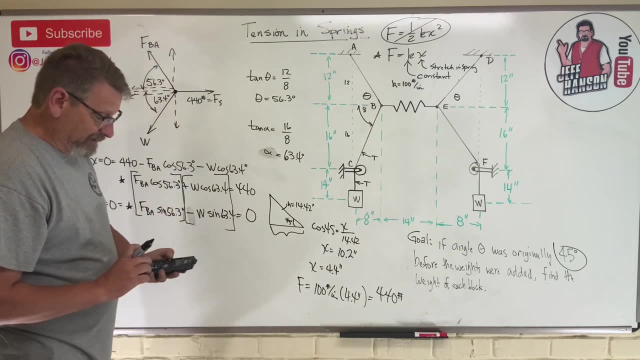 I have this column and then I have this column: Okay, This is unknown Number one, unknown number two, and then constants over there, which is exactly how my TI 36 pro system solver wants it set up. So I'm going to go second system solve two by two click, And then I'm going to enter in. 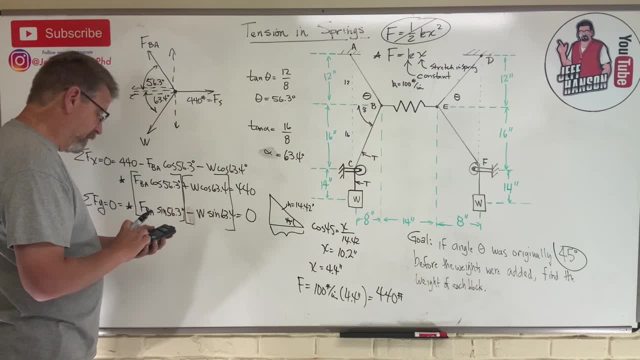 cosine of 56.3. cosine 56.3, enter. Okay, You can just enter the function Minus, minus. What am I going to put? No plus, That's not minus, That's plus Plus. cosine 63.4, cosine 63.4, enter. And then, over here, I'm going to put my 440, 440 enter. 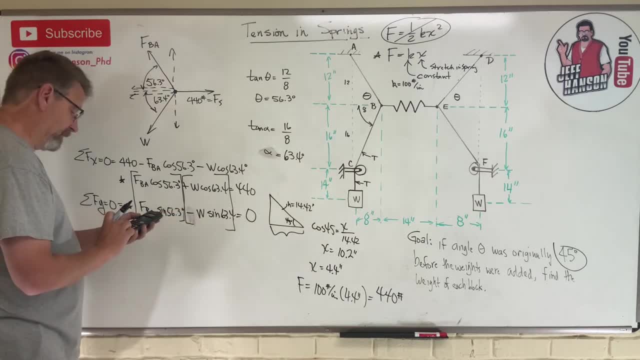 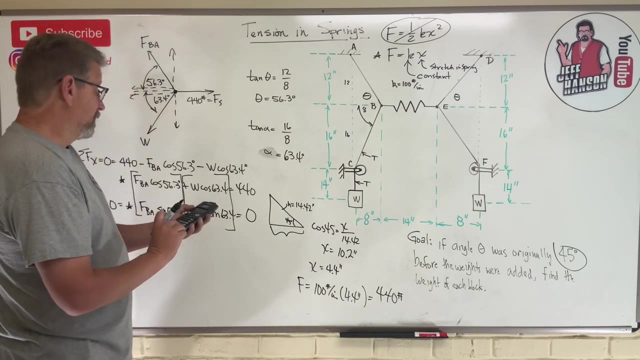 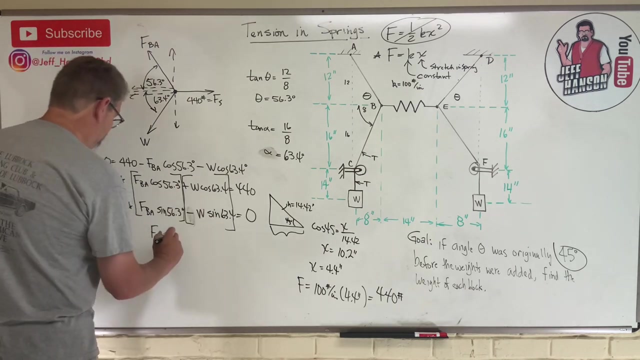 Okay, And then on the next line down, sine 56.3- enter minus. and then sine 63.4- enter zero, enter. And then just click solve Bam. And it gives you the answers, doesn't it? FBA, which is X in my calculator, is 452.9 pounds And W, which is Y in my calculator, right? 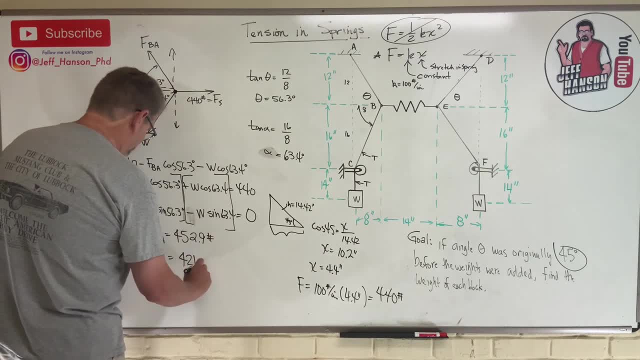 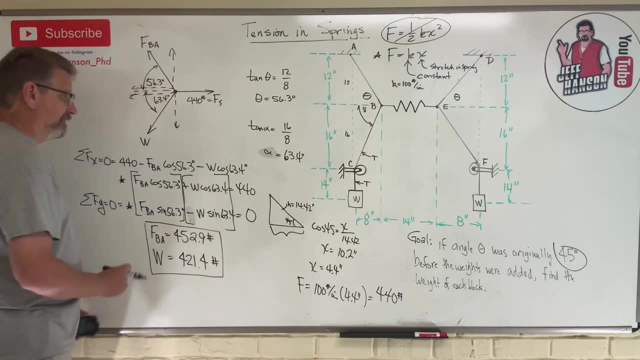 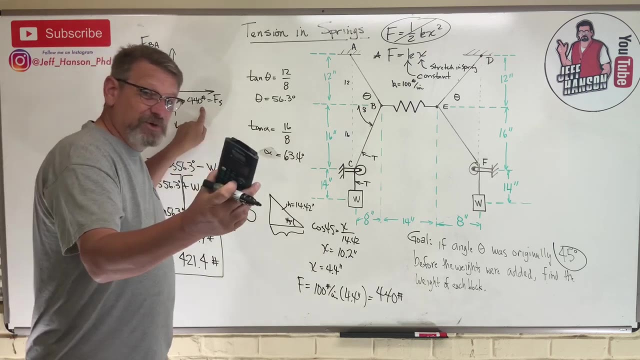 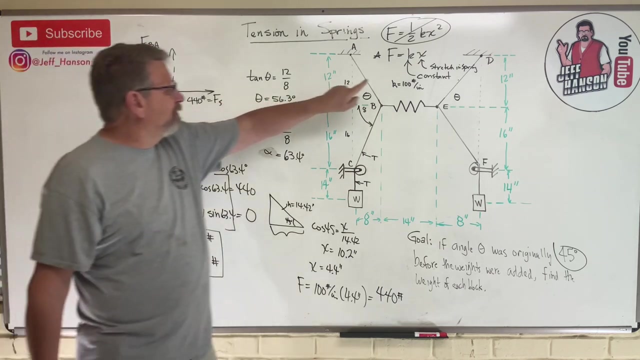 Is 421.4 pounds. Okay, And that is how you do that, right? So the hardest part about this was taking this force in the spring, which was actually given to us, but just in a really weird way. right, We had to do a little bit of a little bit of geometry to come up with the stretch. 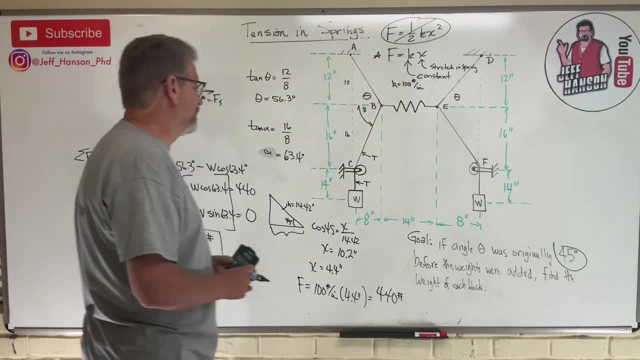 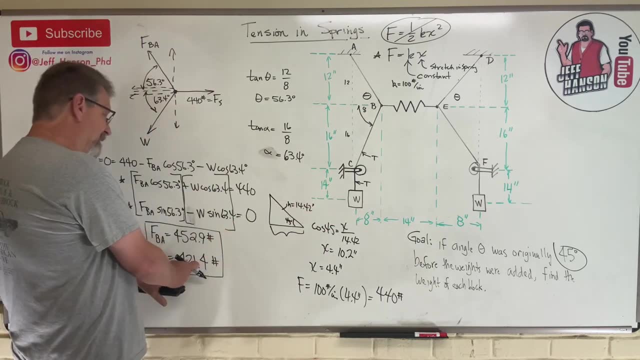 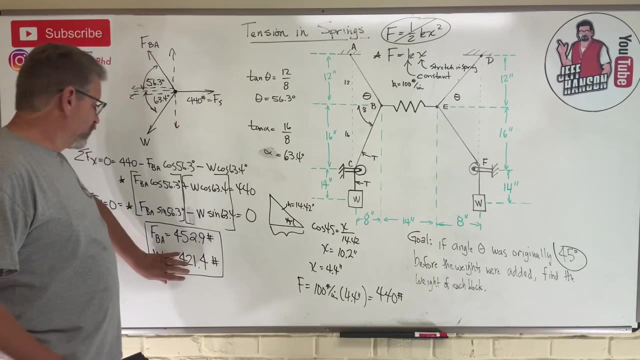 in the spring and multiply by the spring constant to get that force. Now here's a question for you: Do I take this W, do I divide that by two and like that's half of it? No, This W is 421.4.. That W 421.4.. Okay, I hope you don't mess that up. 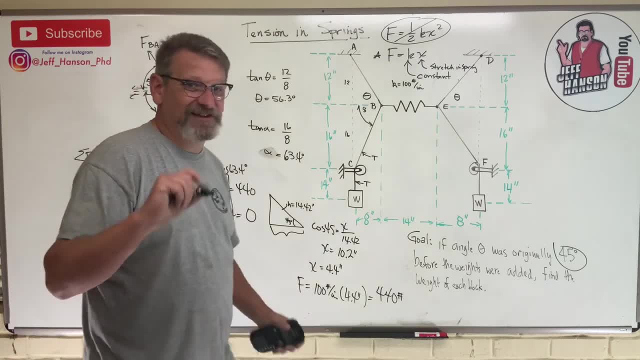 All right, I hope this helps and I'll see you on the next lesson. 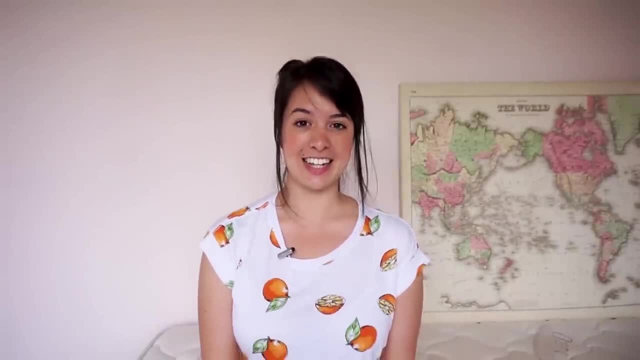 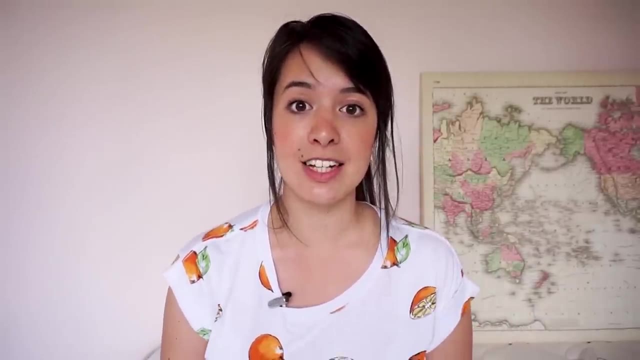 Hello there, lovely to meet you. I've been reading a lot about infinity lately and, guys, it is so cool. We all kind of have a concept of infinity like something that goes on forever and ever and ever. If you try to count, to the biggest number you can think of, you can always add one more. 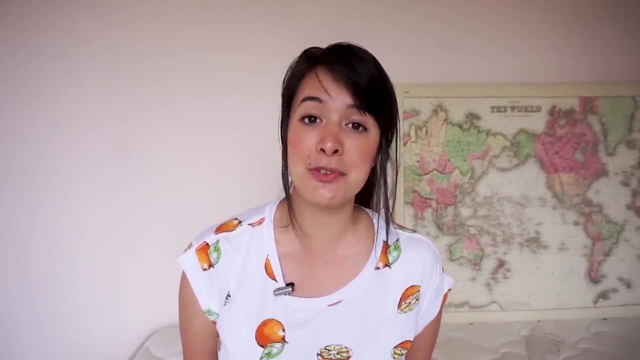 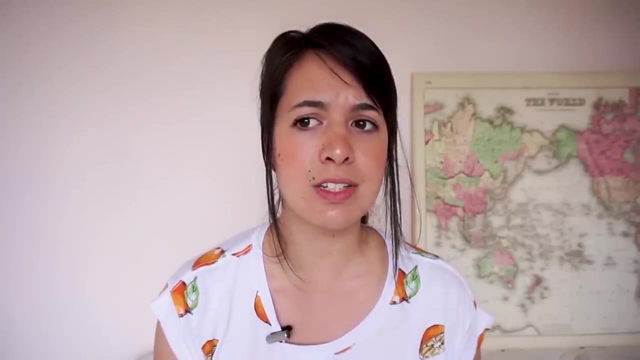 The idea itself isn't that hard to grasp, but when you try to make it rigorous, like mathematics likes to do, that's where things get tricky, It turns out. infinity comes in different sizes. This German guy named George Cantor found that there are different kinds of infinity, and some are bigger. 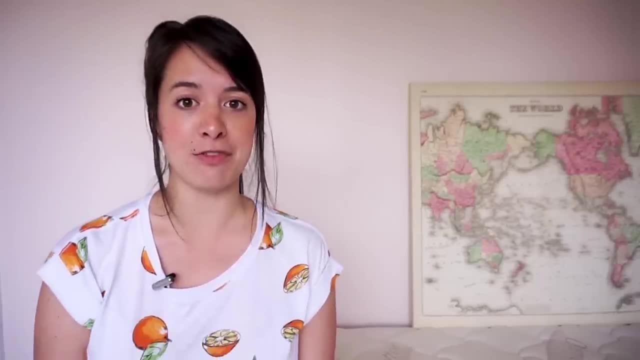 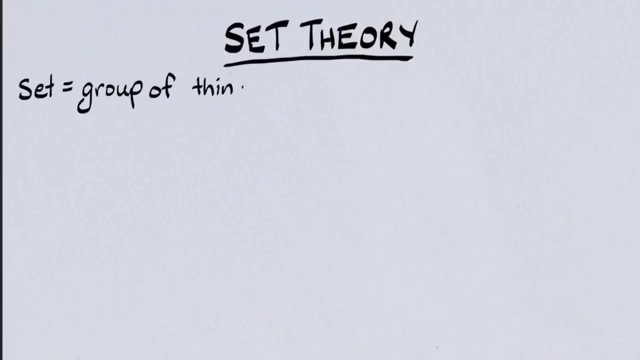 than others. To understand this, we actually need a lot of background information, but the background information is really cool too. We'll start with set theory. A set is basically a group of things. This is a set of four dogs. This is a set of four forks- The number of things or elements in a set. 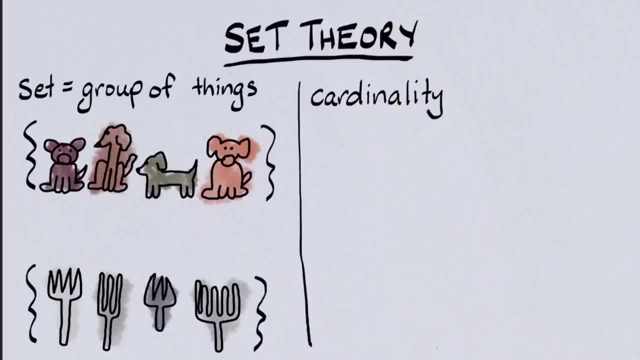 is called its cardinality. so these sets both have a cardinality of four. Now, when two sets have the same cardinality, they are called cardinalities. When two sets have the same cardinality, they are said to be the same size. but size is defined in a bit of a strange way. The normal, intuitive way to